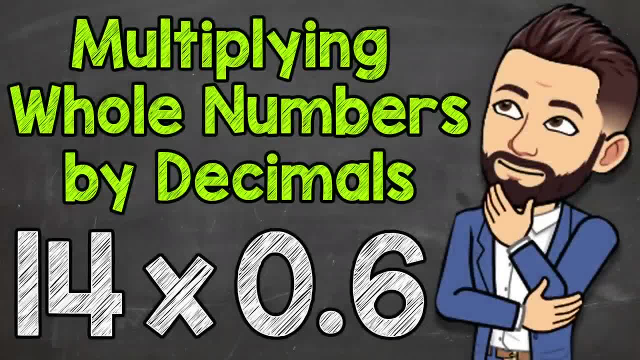 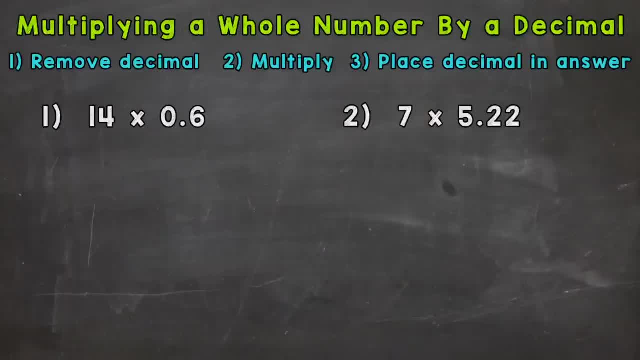 Welcome to Math with Mr J. In this video I'm going to cover how to multiply a whole number by a decimal. So let's jump right into number one, where we have 14 times 6 tenths And the three steps that we're going to take in. 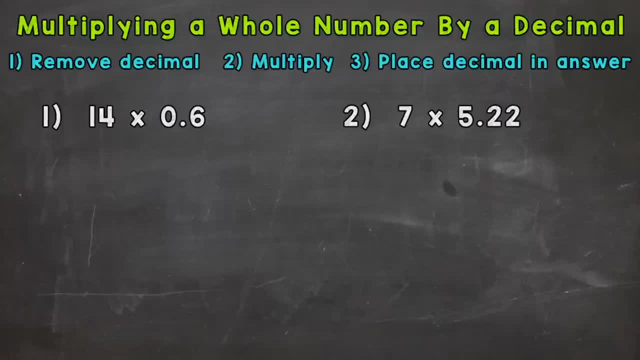 order to solve these two examples correctly, are at the top of your screen And step one says: remove any decimals within that problem And we're going to rewrite the problem without those decimals. So let's rewrite number one as 14 times 6.. So we're removing or forgetting about any decimals. 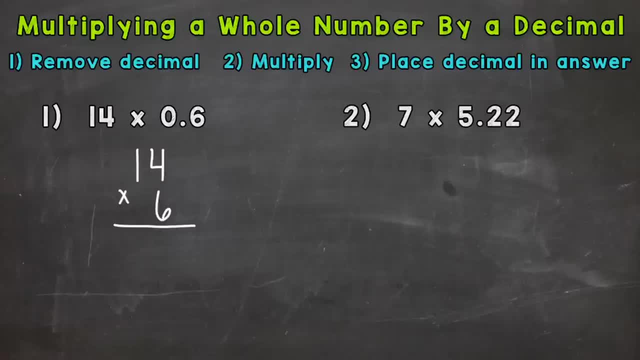 They will come into play later on. in the problem, though. Number two, we multiply or solve just like we would any other multiplication problem involving whole numbers. So 6 times 4 is 24.. 6 times 1 is 6, plus that 2 is 8.. So we get an answer of 84, but we're not quite done yet. 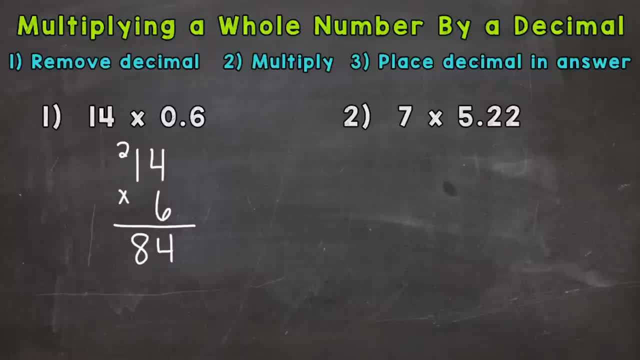 Step three, we need to place the decimal in our answer And we do that by looking at the original problem and seeing how many digits are to the right or are behind a decimal, However you like thinking about it, And we have 1. This 6 here, And I like circling any digits to the right of a. 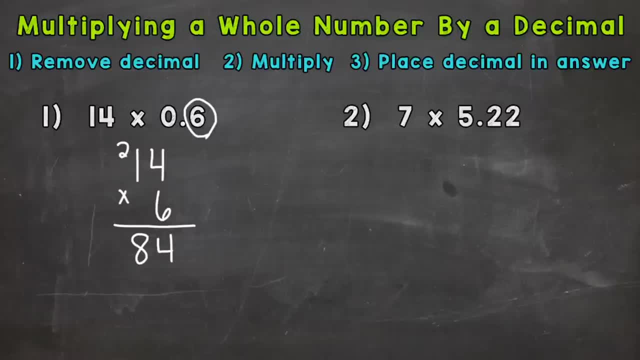 decimal or behind. That way I make sure I include everything. So we have one digit behind a decimal. That means our answer has to have one digit behind it. So that means our answer has to have one digit behind the decimal. So this 4 will be our one digit And we can place our decimal right there. 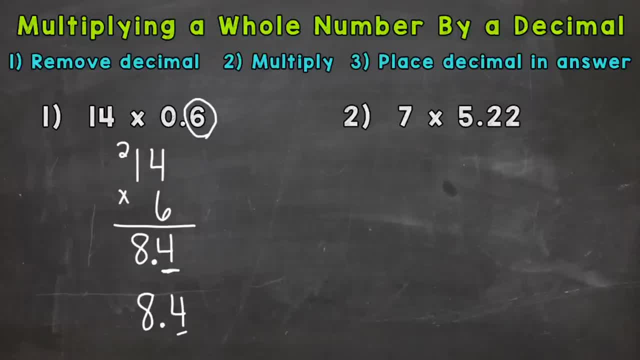 So we have eight and four tenths as our answer. Another way of thinking about it: we had 84 as our answer. So for every whole number the decimal is at the end. So we can bring our decimal in once. That way it gives us one digit behind the decimal, Or you can just: 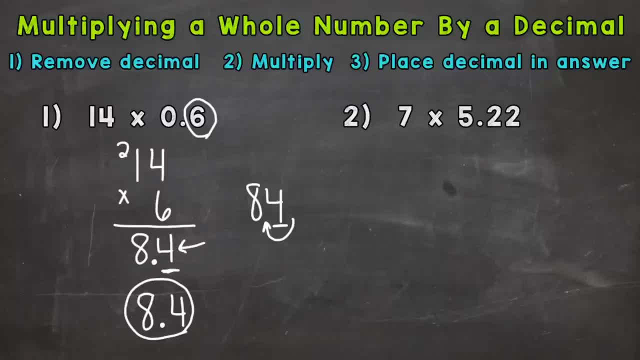 umhow I did right here and now. my last amount is 2.. I'm just going to give it the other way around: right here kind of counted how many digits i needed and placed the decimal accordingly, whatever works best for you. so on to number two here, where we have seven times five and twenty two hundredths. 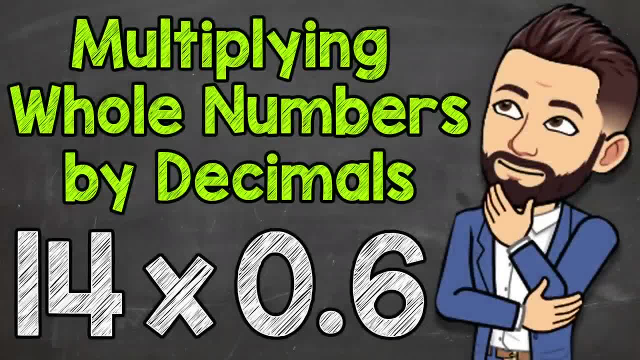 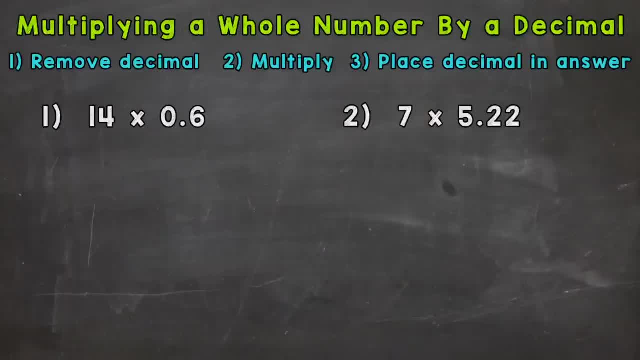 Welcome to Math with Mr J. In this video I'm going to cover how to multiply a whole number by a decimal. So let's jump right into number one, where we have 14 times 6 tenths And the three steps that we're going to take in. 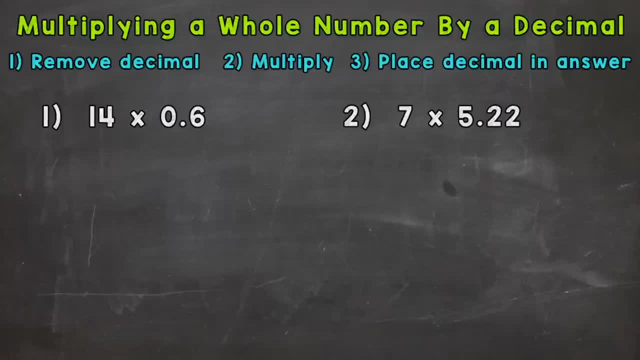 order to solve these two examples correctly, are at the top of your screen And step one says: remove any decimals within that problem And we're going to rewrite the problem without those decimals. So let's rewrite number one as 14 times 6.. So we're removing or forgetting about any decimals. 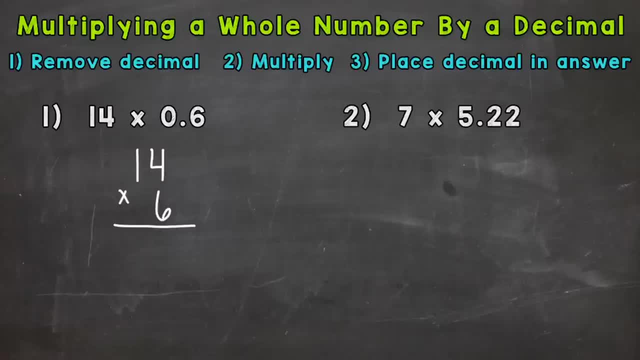 They will come into play later on. in the problem, though. Number two, we multiply or solve just like we would any other multiplication problem involving whole numbers. So 6 times 4 is 24.. 6 times 1 is 6, plus that 2 is 8.. So we get an answer of 84, but we're not quite done yet. 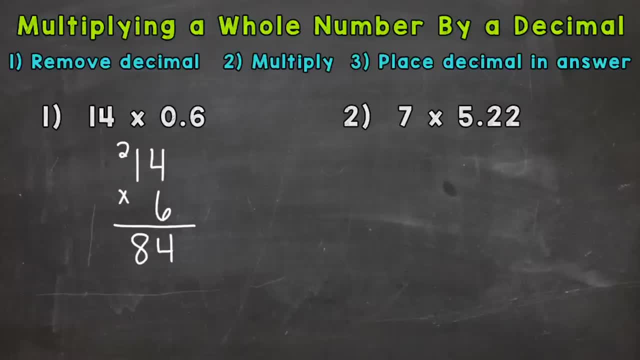 Step three: we need to place the decimal in our answer And we do that by looking at the original problem and seeing how many digits are to the right or are behind a decimal, However you like thinking about it, And we have one, this six, here, And I like 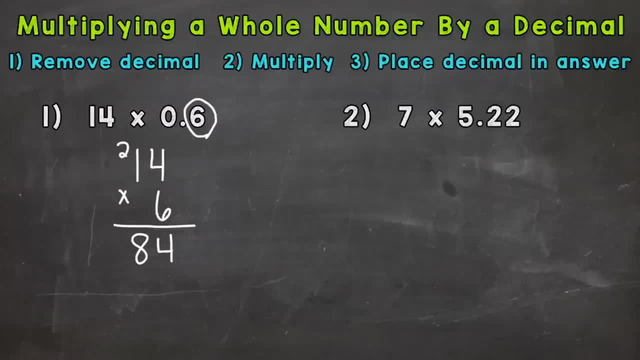 circling any digits to the right of a decimal or behind. That way I make sure I include everything. So we have one digit behind a decimal. That means our answer has to have one behind the decimal. so this four will be our one digit and we can place our decimal right there. 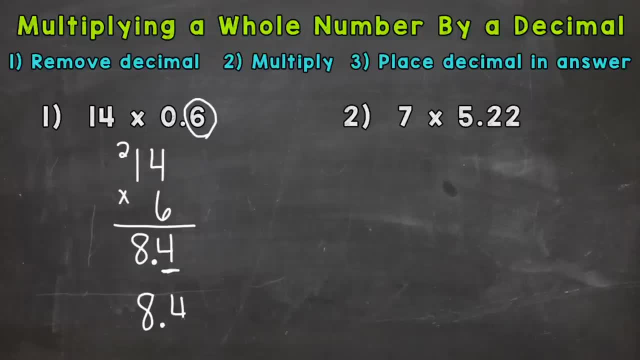 so we have eight and four tenths as our answer. another way of thinking about it: we had 84 as our answer. so for every whole number the decimal is at the end. so we can bring our decimal in once. that way it gives us one digit behind the decimal. or you can just how I did, right here. 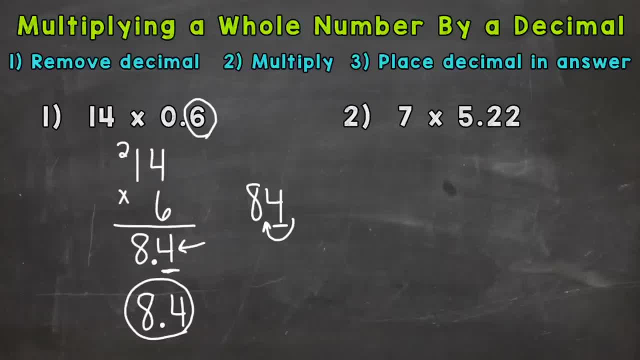 kind of counted how many digits I needed and placed the decimal accordingly, whatever works best for you. so on to number two here, where we have seven times five and twenty two hundredths. first step: remove any decimals and rewrite the problem. so we get seven times 522. now, when it